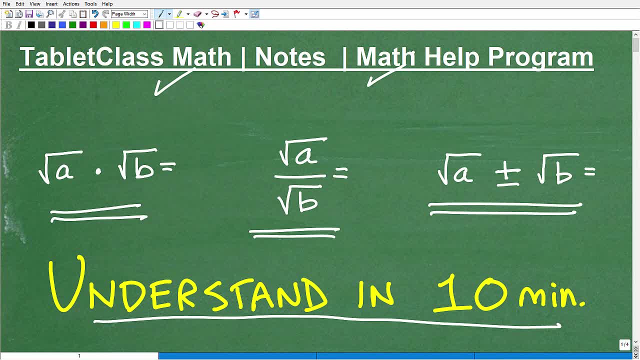 And over several years I've constructed what I like to believe is one of the best online math help programs there is. Of course, I'll let you be the judge of that. You can check out my math help program by following the link in the description of this video. But basically I have 100 plus different math courses, ranging from pre-algebra, algebra one, geometry, algebra two. I'm going to be launching pre-calculus here shortly. I'm very excited about that, But I also do a lot in the area of test preparation. So if you're studying for the GE, 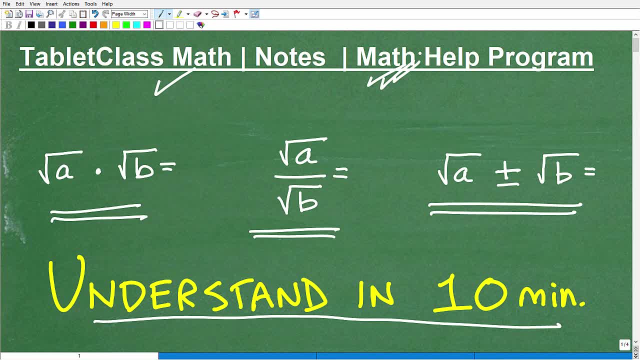 D, SAT, ACT, GRE, GMAT, ASVAB, ACCUPLACER, CLEP exam, ALEKS exam, maybe a teacher certification exam. All those exams I mentioned have a lot of math on them And if you don't do well in the math section, you don't do well on the exam. So if you're studying for a particular exam, just go to my website And you can check out my full course catalog. I should have the test you're studying for If I do not drop me a line, and it will help you out the best I can. I also do a lot with independent learners, like homeschooling. 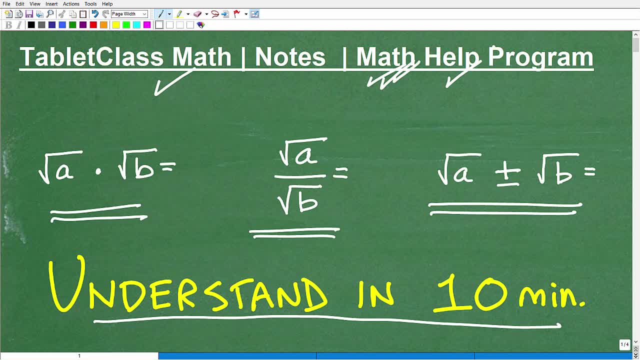 So if you homeschool, I have a great homeschool learning system. And then, lastly, I help those of you that are just having a tough time in your current math course. Now, one thing I cannot do for you that you must do for yourself if you're serious about improving in mathematics, and that is taking great math notes. So over decades of teaching math- really- I think this is the secret to doing very well in mathematics- is note taking. I've just seen this over and over again: Those students that take great notes almost always have great math grades, And the reverse is true. 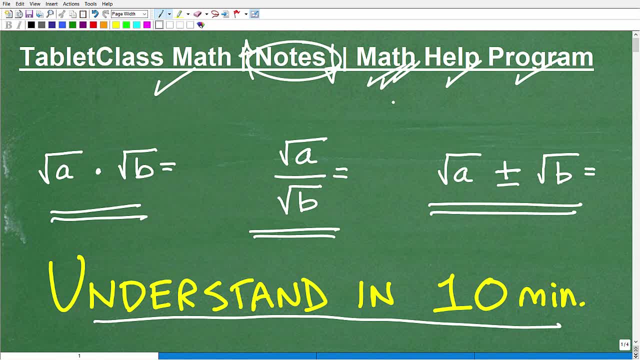 Those students who blow off their notes, like I did. way back in the good old 1980s, I was like, yeah, note taking, Yeah, whatever, And always ended up with grades like C minus. It wasn't until later on in college and after the Marine Corps, where I got some discipline And I said: you know what? there's only one way to learn something. You got to pay attention, right, You got to stay focused. So note taking is that activity that will help you out. Now, as you're improving, you still need something to study for. 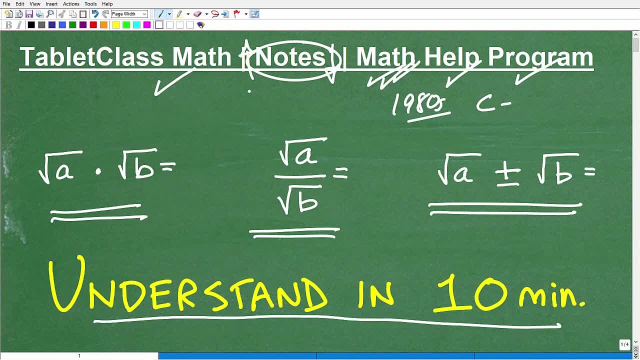 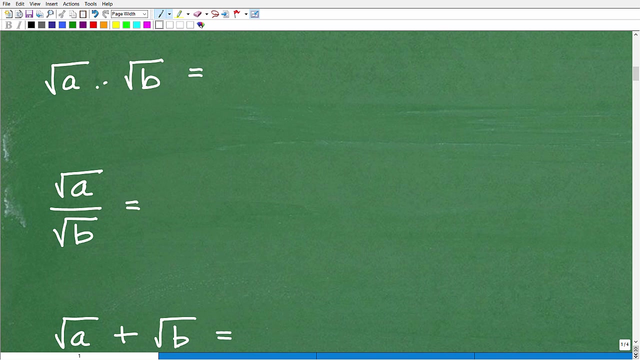 Study from. So I offer detailed, comprehensive math notes to include pre-algebra, algebra one, geometry, algebra two and trigonometry. You can find the links to those notes in the description of this video. All right, So let's get into these operations with square roots, And I'm going to try to keep this about 10 minutes, We'll see how I do. All right, So let's go to the first one. So we're trying to multiply, or when we multiply two square roots, So square root of A times the square root of B, That's equal to the square root of B. 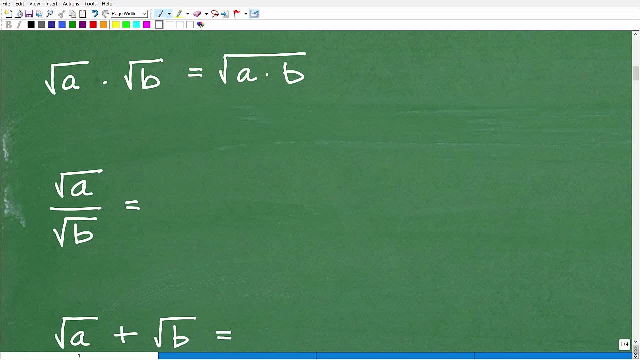 Okay, So you want to write that down in your notes? if you don't have that? So let's just take a look at a basic example: Square root of three times the square root of two. Okay, So how can I do this problem? Well, you just write one big square root- Let me simplify this a little better here- And we just go: okay, this is going to be square root of three times two, which, of course, is the square root of six. Okay Now, 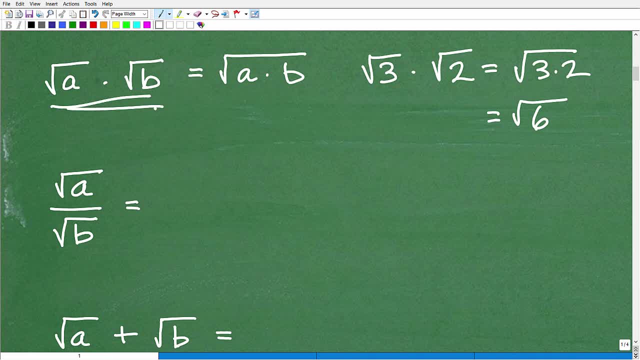 this property plays a very important part for us to simplify radicals. Let me give you another example here. Okay, So, if you understand this, this is pretty straightforward. Let's take a look at doing this in reverse, because this is very, very important. Let's say, I have the square root, Let me write it here: Square root of 20.. Okay, So you say, okay, square root of 20.. Well, how can I simplify this square root? And you need to know how to do this as well. Well, 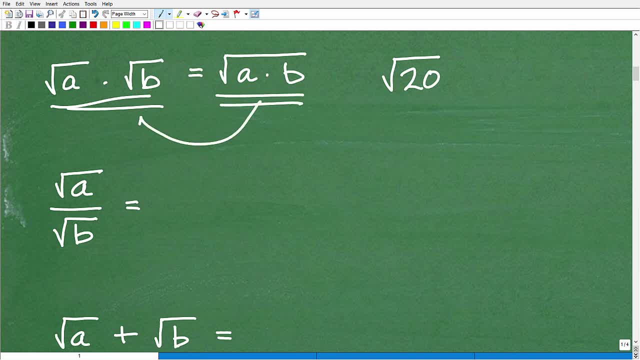 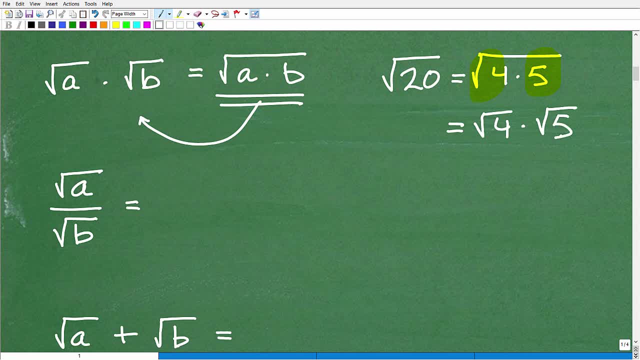 times the square root of 5.. Now, why would I want to do that? Well, because I can take the square root of this nice little, what we call perfect square. The square root of 2 is positive, negative 2.. We'll just write a little 2 here, 2 square root of 5, and there you go. Okay, so when you're faced, 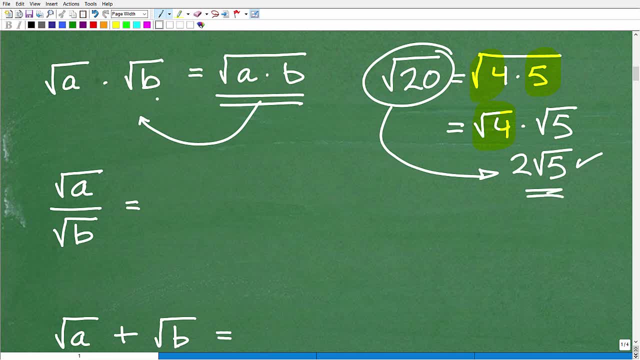 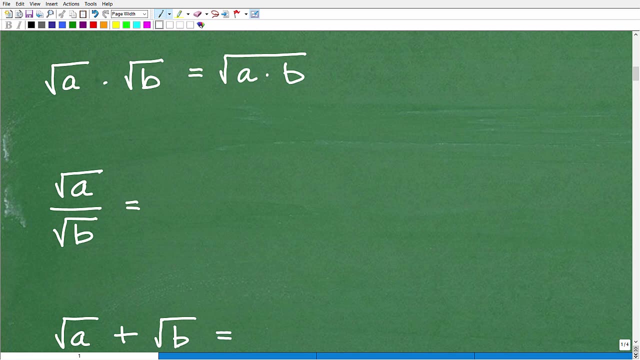 with a radical like this, you need to simplify by using this particular property backwards. Okay, all right, so I got to get 10 minutes. Maybe I've already used 5.. Let me go ahead and continue on. Okay, just one little thought here as well, If you have additional questions on this or you want to. 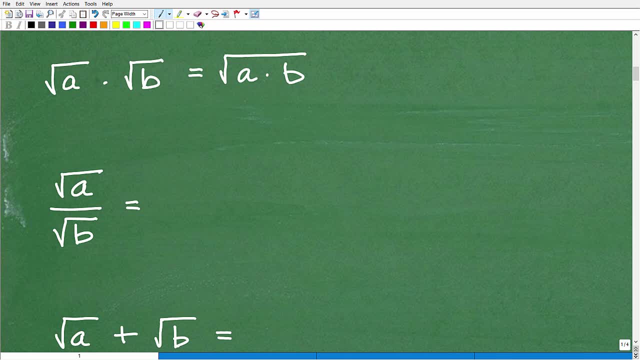 continue to learn this. a couple suggestions. I have tons of videos on my YouTube channel in my algebra playlist on square roots. You can check those out. or, better yet, just join my algebra course in my math help program. All right, so let's talk about the division of radicals. So 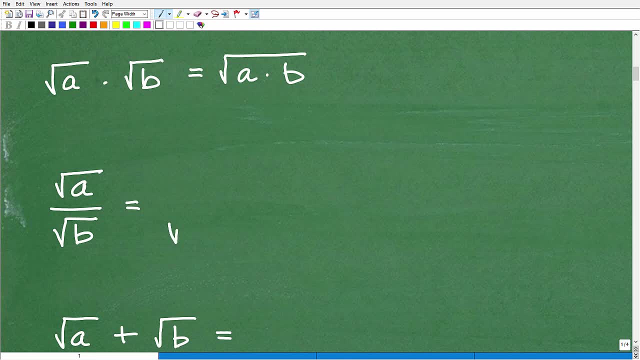 we have the square root of a Divided by the square root of b. Well, guess what? You could just have one big square root of a over b. Okay, it's very similar to this. Let's take a look at an example. What if I have the? 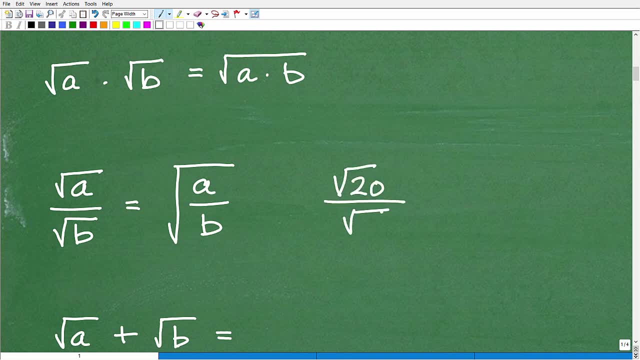 square root of 20, and I'm dividing it by the square root of 5? Okay, so this right here, in and of itself, we're like. well, I don't really like this, By the way. you never want to have. 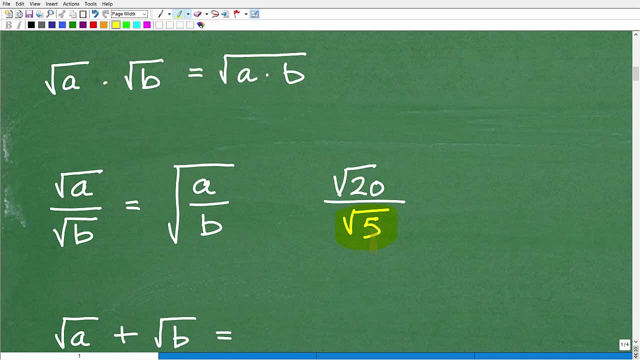 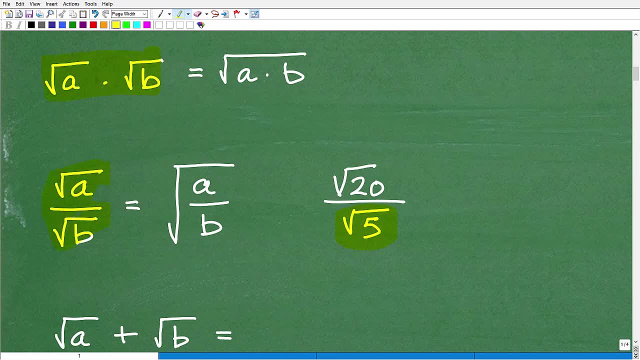 I'm just focusing in on these basic math operations, multiplication, division, etc. But here I could say: well, I have the square root of 20 divided by the square root of 5.. We could just have one big radical 20 divided by 5.. And this little square root symbol is also called a. 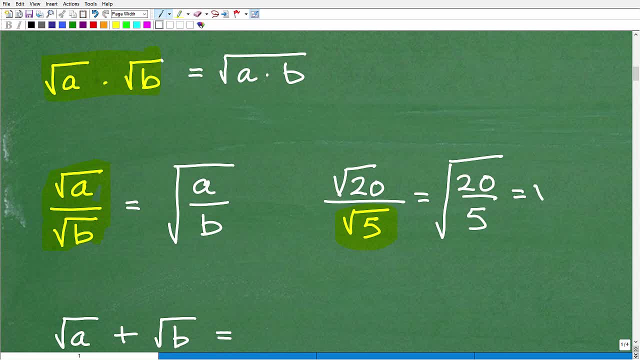 radical, if you didn't know that. And 20 divided by 5 is what? Well, that's the square root of 4, and the square root of 4 is 2.. Really, square root of 4, but we are talking about square roots here- is really positive and 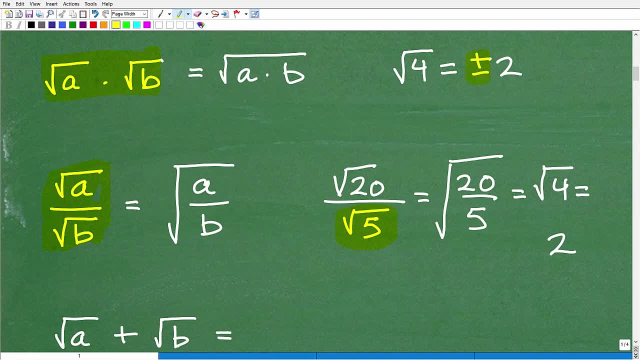 negative, 2.. All right, so you should get in the habit of writing both this little positive and negative there, because 2 times 2, positive, 2 times positive 2 is 4.. And negative, 2 times negative 2 is also positive 4.. Okay, so when you take the square root of a real number, 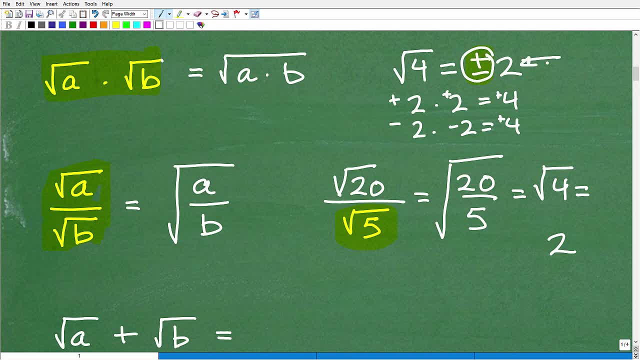 don't forget this little positive and negative sign. It's very important. Okay, All right. so, anyways, that's the division of two square roots or two radicals. Okay, All right. so if you understand these two properties so far, then you know that's very good, Okay. 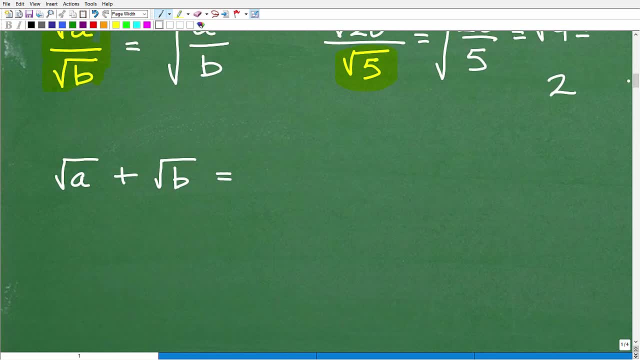 you're like you're going to walk away from this little video with an increased knowledge of this stuff for sure. All right, let's talk about adding and subtracting. So this property here I'm going to talk about next is for both addition and subtraction of radicals. 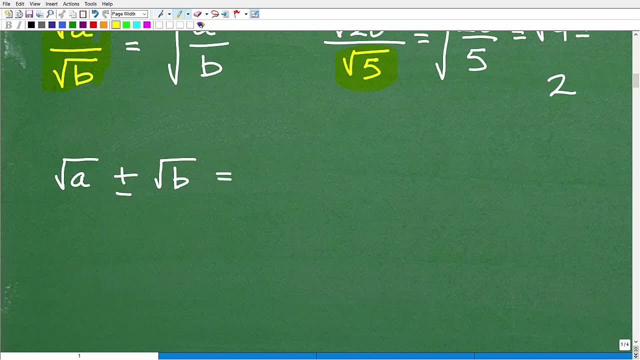 Now this one is a little bit different. Okay, You can only add these here if these two are the same. Okay, so let me give you an example. It's easier to show to show this. So if I have 3, 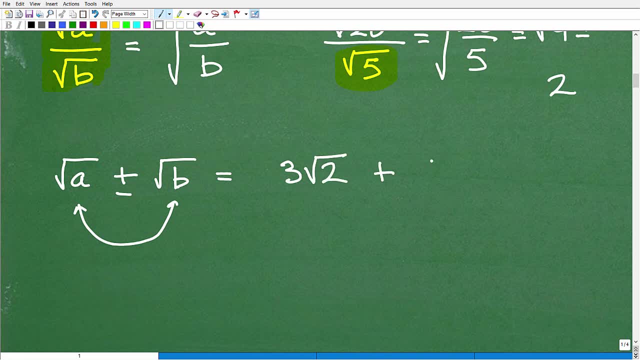 radical 2 or square root of 2 plus 5 square root of 2, I can do this problem. I'm going to go, I'm going to do this here in a second, But if I have 3 square root of 2 plus 5 square root of 2,, 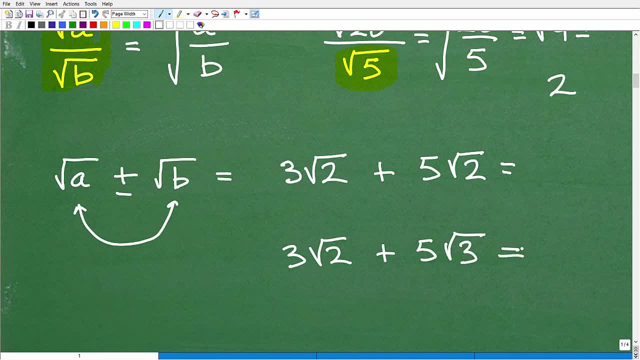 this I cannot do. Okay, Now you can add or subtract square root terms, Okay Expressions. If the these here, these square roots, are exactly the same, Okay, They have to be exactly the same. In other words, this is the square root of 2.. This is a square root of 2.. So I just add these. 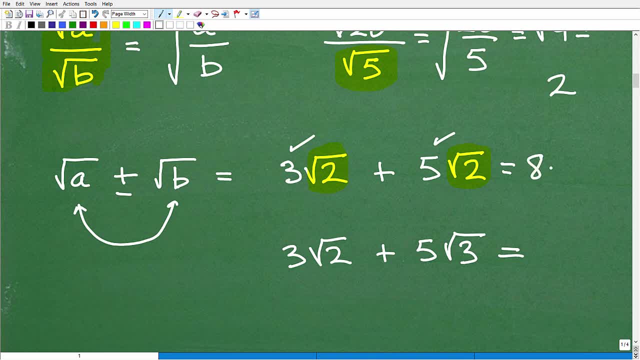 numbers here: 3 and 5.. So this is 8 square root of 2.. Okay, Now this one here: 3 square root of 2 plus 5 square root of 3, I cannot do the this problem. This is as fully simplified I'm done. 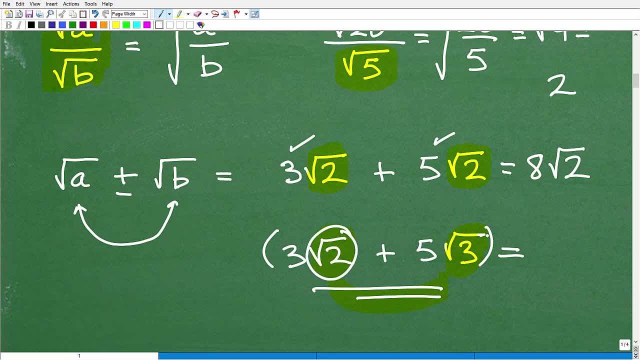 right here. Okay, It's as fully simplified as I can go, because these two are different. This is very much like an algebra: when you're combining like terms like 2x, I can combine with 5x, because these are exactly the same Same thing here. Now let's go back to this problem. I have 3 square. 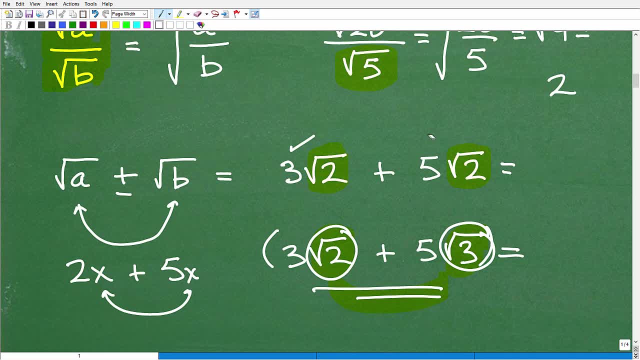 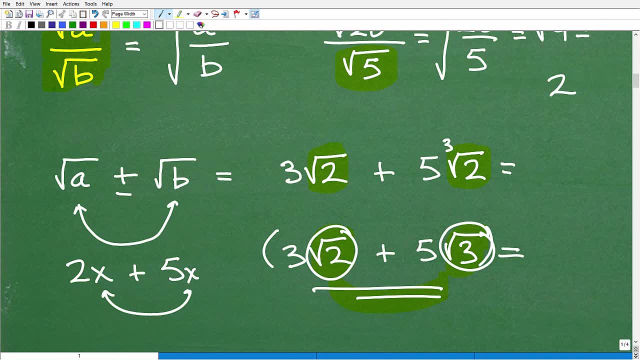 times the cube root of 2.. Could I do this? No, I cannot because, again, these two are not exactly the same, They're different. So this would just be the final answer. Okay, So I don't know if I'm. 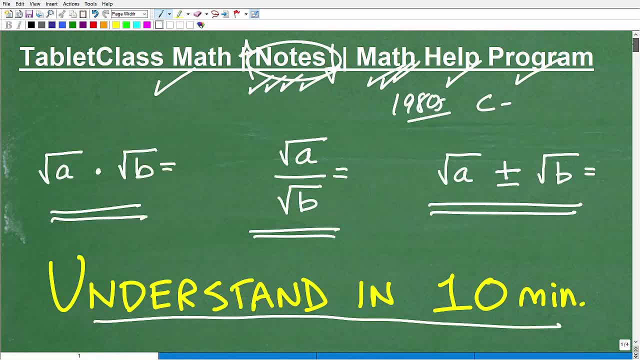 at 10 minutes, over 10 minutes. but listen, you know, my thing is I try to have these little catchy titles to kind of draw you in, you know. but I always want you to walk away from my videos learning something, Okay, And if you, you know, feeling like, Hey, you know, I learned a lot. 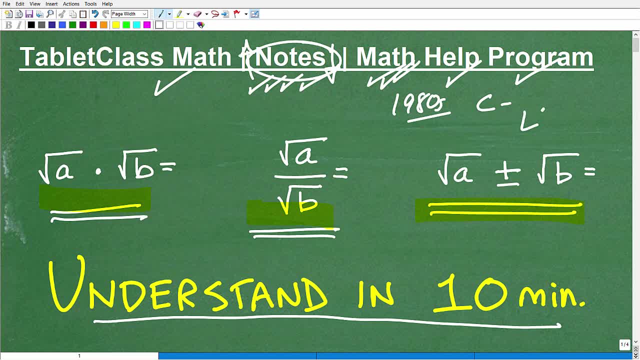 in a short period of time. Well then, I did my job. And if that is the case, please do myself a favor and smash that like button. Okay, And if you're not a subscriber to my channel, hopefully you'll consider subscribing. I've been on YouTube for over 10 years. I have over a thousand plus. 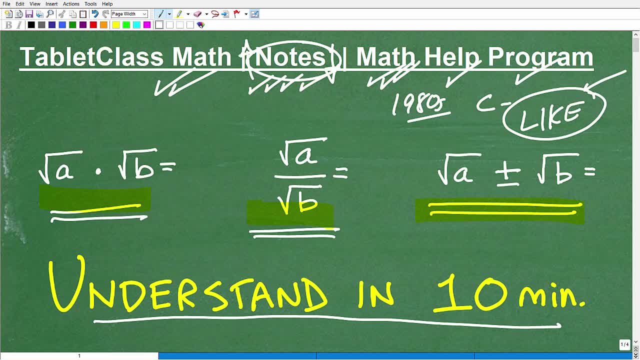 videos- basic to advanced math organized- and various playlists on my channel. They're there for you. My passion is to try to teach math in a clear and understandable way. So if you'd like my teaching style, I have a ton of you know. 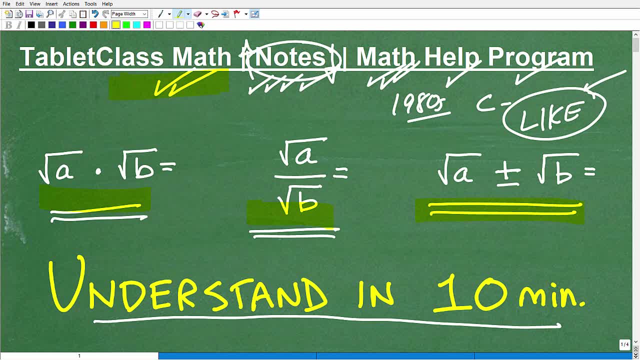 resources and videos, and I'm posting new content all the time, But, again, my best math help will be within my math help program. Okay, So, with that being said, I definitely wish you all the best in your mathematics adventures. Thank you for your time and have a great day.